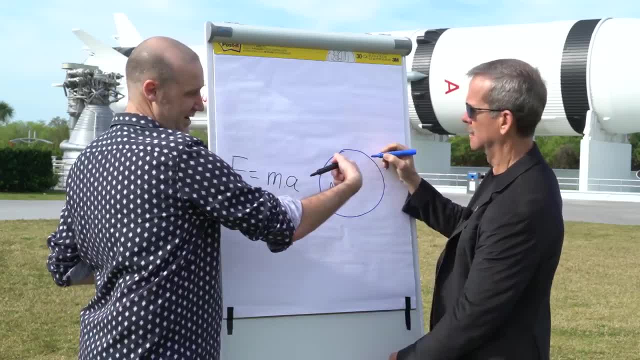 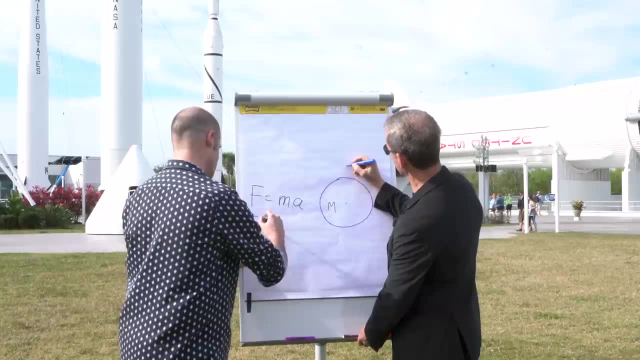 That seems about right. All right, So you orbit. This was the North Pole looking down. North Pole looking down, You orbit around with: Yeah, that's right, Okay, Okay, Yeah, we go with the rotation of the Earth. So I'll draw myself as a dot here. 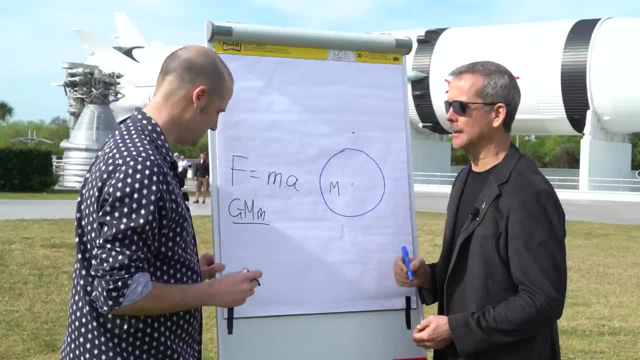 I've given you mass little m. if that's okay, That's fine. I'm happy with little m. Good, good, good, All right. And how far up are we talking here? Well, we're about 400 kilometers. 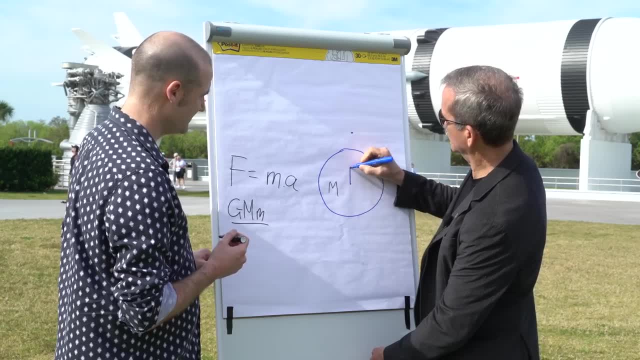 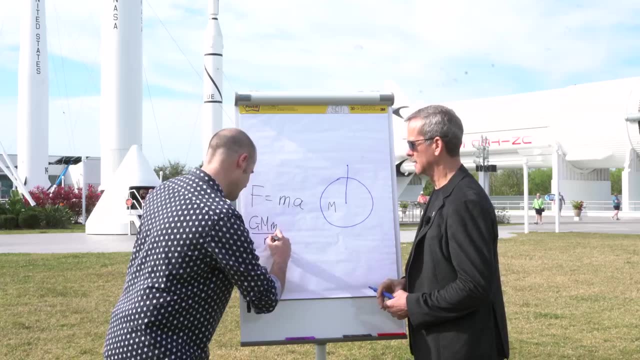 Above the surface, But of course we want to measure it from the center of the Earth So we can put this whole thing right out to there. So it's the radius of the Earth plus our orbital altitude. Okay, Let's call the whole thing R. 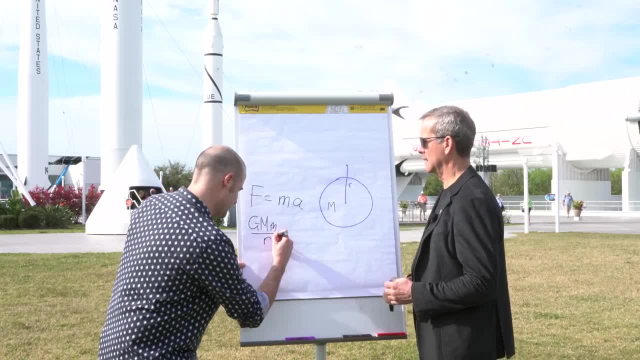 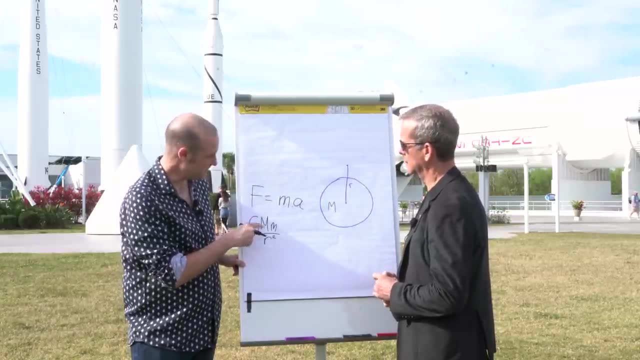 R. Okay, All right, Oh sorry, R squared. So I've just put in the classic gravitational force, the gravitational constant: G mass of the Earth, M mass of Chris and everything else That's keeping you alive, Okay. 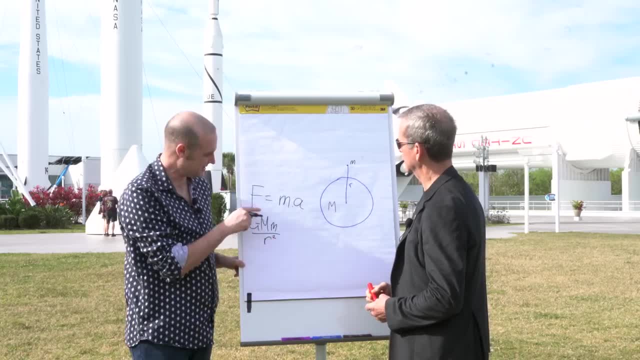 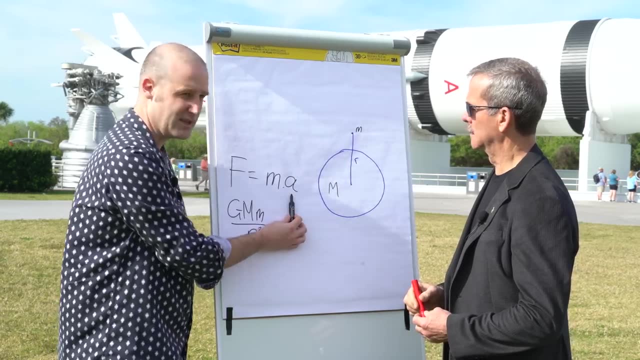 Up there. And then this is our distance: R squared. So that gives us the force that the Earth is pulling you down, And we now need to work out. well, we know M. Well, we've got M. We need to know the acceleration. 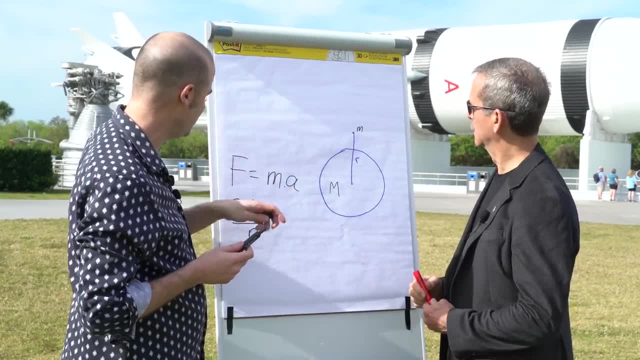 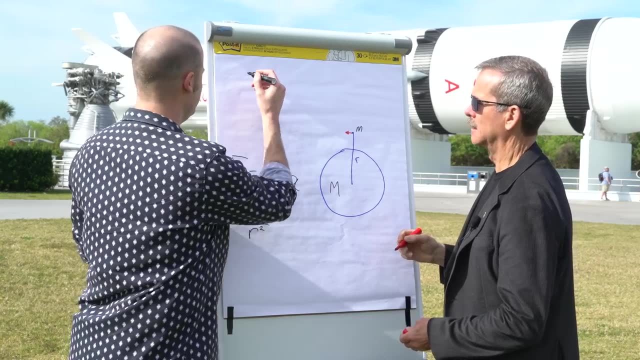 So to do that, let's start with the velocity you're traveling. Okay, So I'm going this way at a certain speed, a certain velocity, right, Okay, Should we call that? do you want to call that V? Sure, Which V? 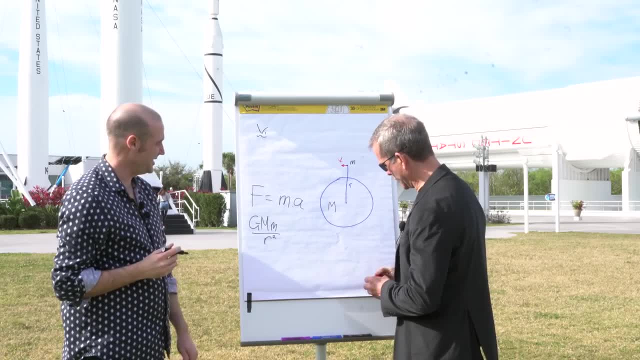 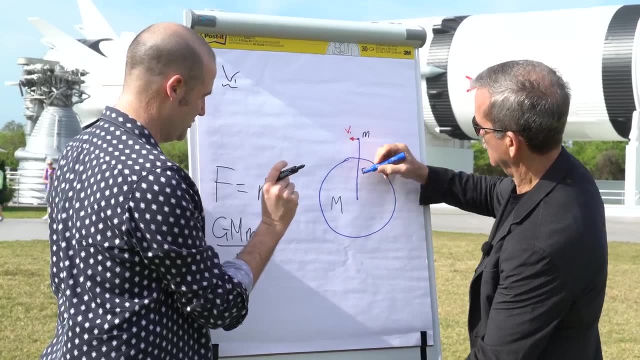 V1.. And it's a vector, So I'm going to put a squiggly line under there. Okay, That's fine. I'm a bit of a perfectionist. We're now going to have a look at you very small moment of time in the future. 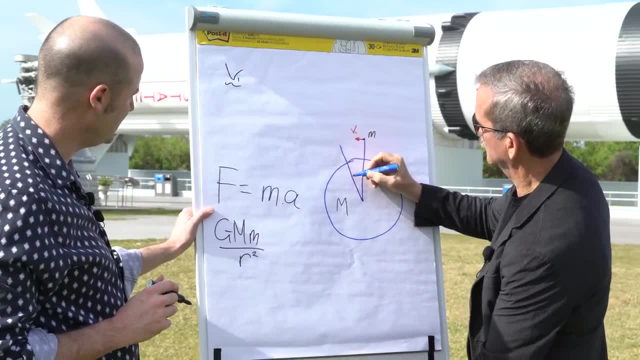 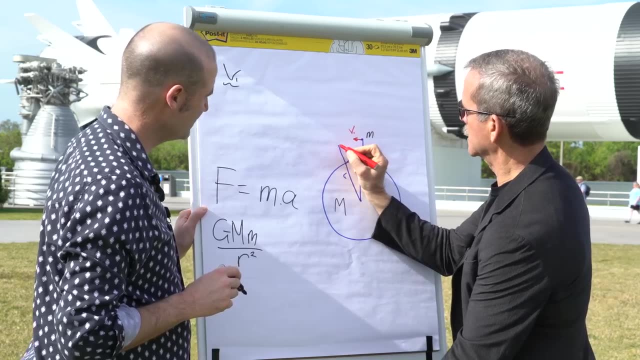 Okay, So over here somewhere, same radius, That's it. Okay, That's kind of the trick to staying in orbit is this has to stay the same. Uh, yep, Basically, And now we want another one here, Yep. 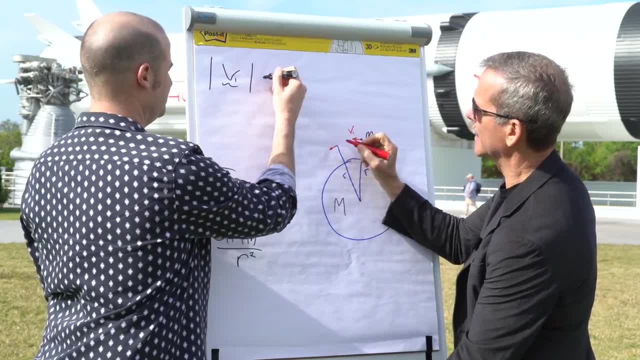 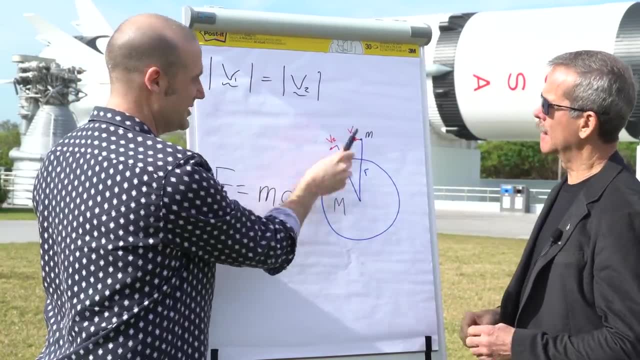 Okay, Always parallel to the Earth's surface. And that's another V, Let's go V2.. Yeah, Okay, Okay, And so I've done up here. I've just written that their magnitudes are the same, Yep, And so actually I'm just going to call it V for shorthand, because you don't. 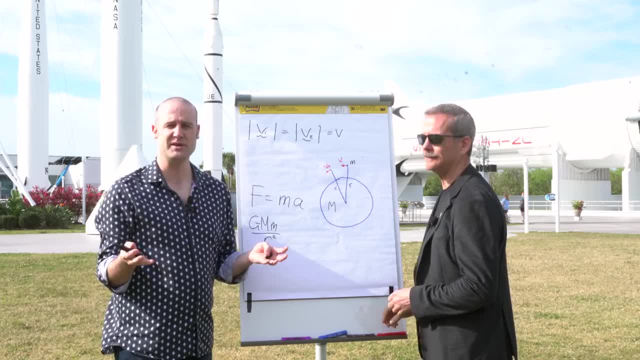 want your speed to slow down, Correct, Correct, I guess that's kind of the definition of being in orbit. Uh, yep, You're not getting lower, You're not slowing down, We're just going like the moon, round and round and round. 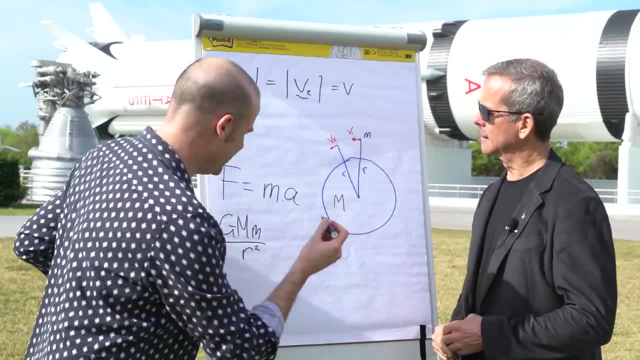 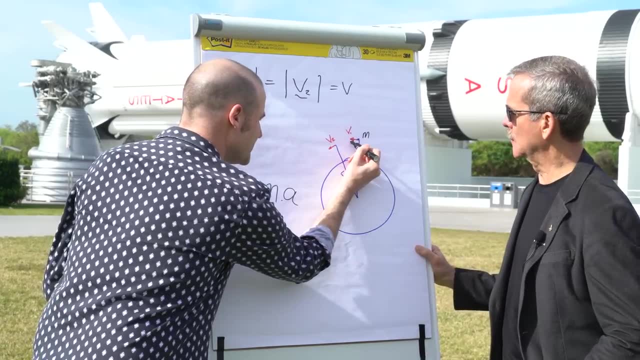 Perfect, Okay. So now I'm going to add in a little angle here: This is going to be theta, Theta, All right, And then we've got the distance you've traveled, So you've gone from there to there, Yep. 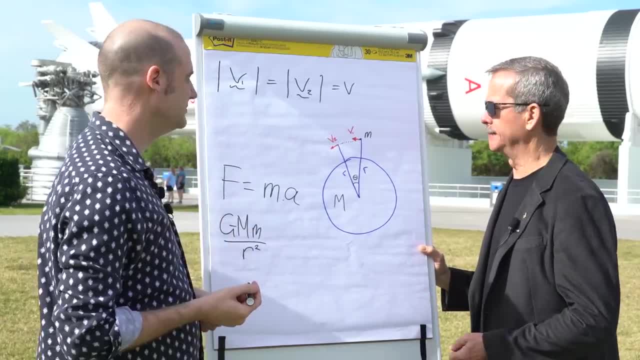 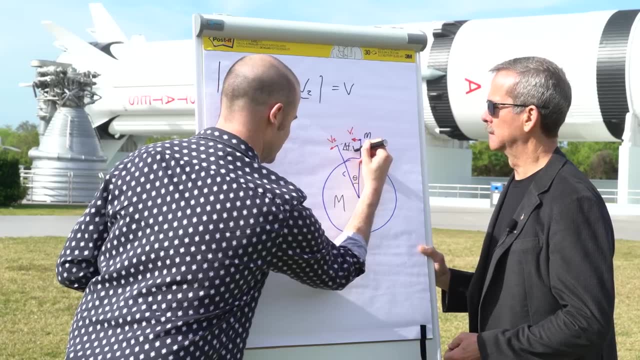 And that's going to be, I mean Proportion at the time. Yeah, So that's, let's say, over this tiny angle, tiny amount of t. So I'm going to put in delta t times, Whatever velocity you're moving at. 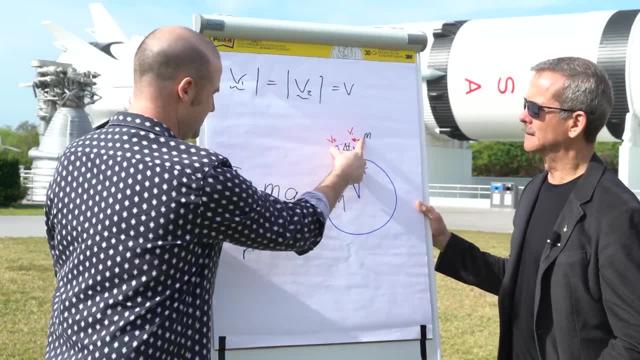 Sure, We're now going to move these vectors and I'm going to redraw them over here, So I'm going to borrow your red, All right? Okay, So I'm going to bring V1 over here and zoom in on it like that. 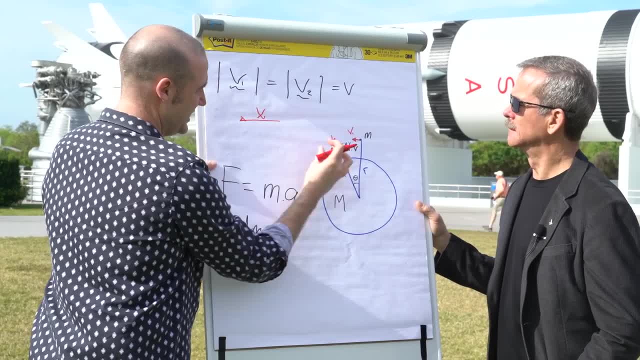 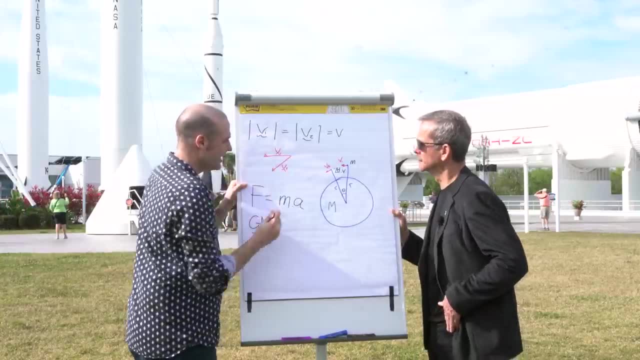 That's a V1 vector, And then I've just moved that straight across And this one is now on an angle down. So if I bring it over there, that's V2.. Yep, And as you go around, I guess by the time you come all the way back to where you started. 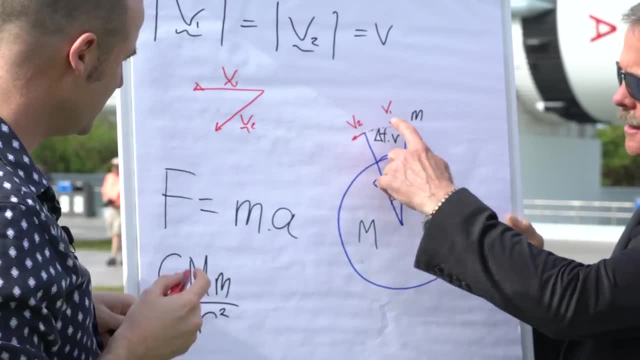 velocity is once again going perpendicular. Yeah, At our altitude it takes about 92 minutes to go all the way around. All right, 92 minutes per lap, Yep Per lap, And then theta will go through a full 360. 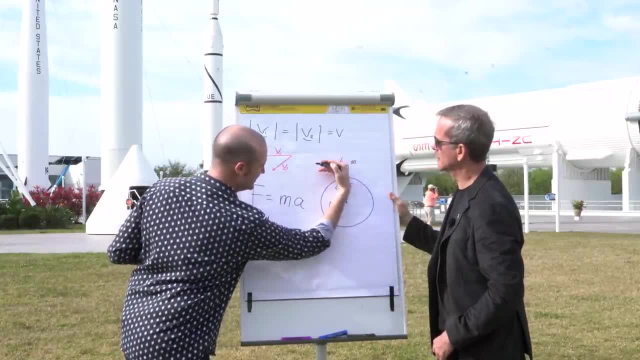 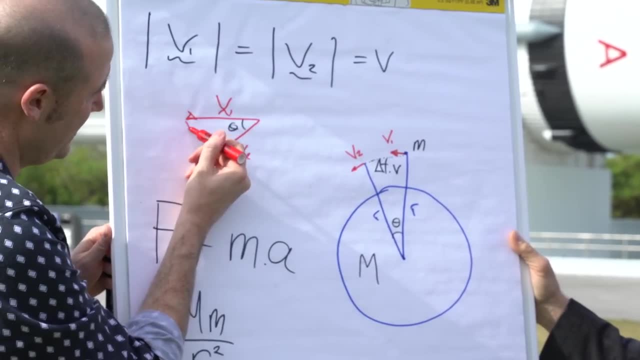 360.. So actually this angle, this has just tipped your V down Right. It's actually gone down by theta: Yep, Same amount Yep, And now that's the difference there. So I don't know if you do a lot of vectors. 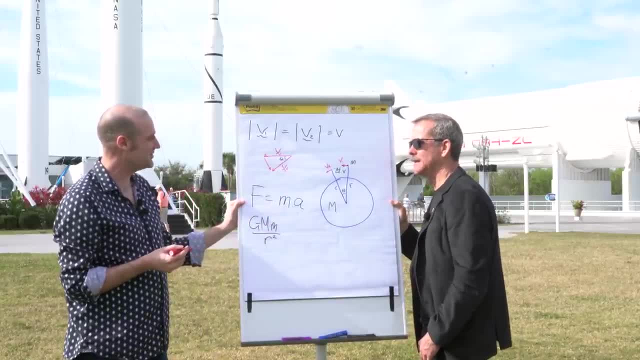 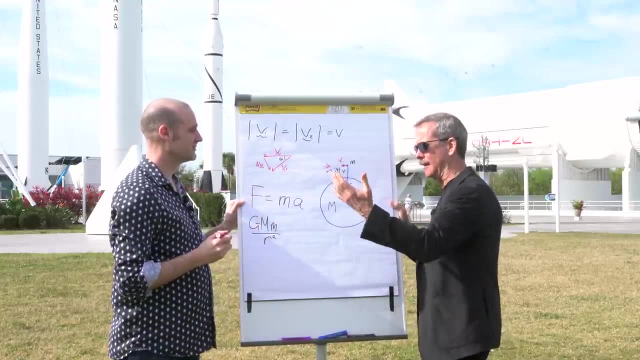 as an astronaut Do you have to do much math? as an astronaut, You have to understand how it all works. but real time you're mostly just solving the practicality. Yeah, Like how do I get my spaceship from here to there And we let the computer do the burn? 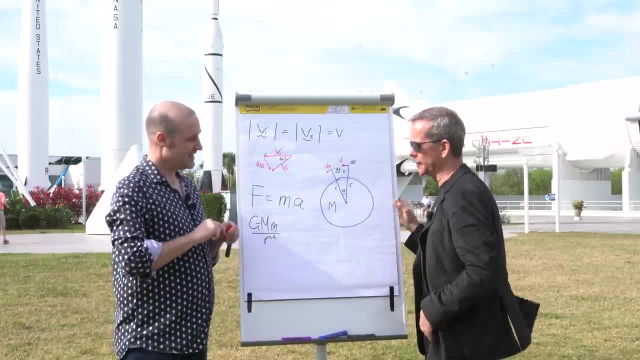 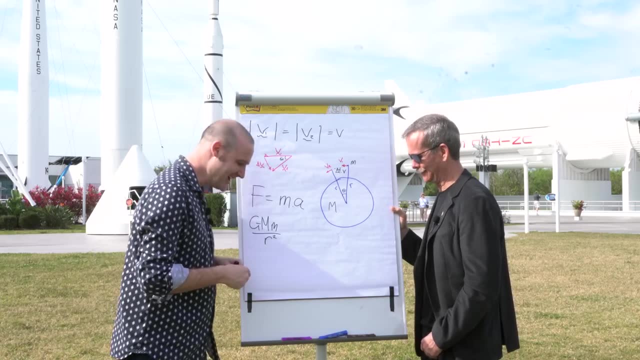 calculations, You have to have a sense of how it all is supposed to make most of the work. but we don't real time do a lot of math in public, So I'm watching and bowing to your expertise. Well, no, no, I mean, I guess you've got a very pragmatic. you know the math. 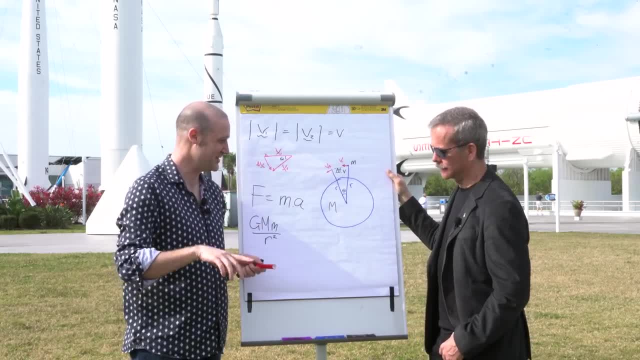 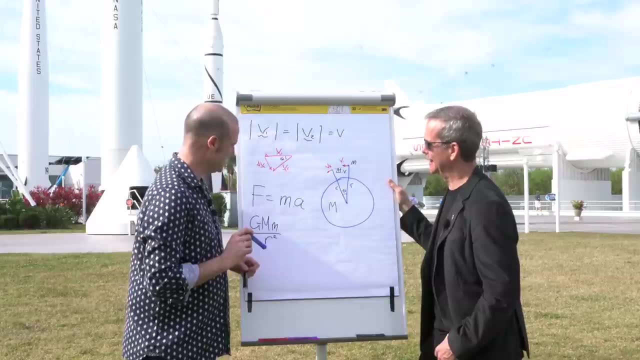 so you understand what's meant to be happening, Yeah, And then you trust the computers and just kind of sense check as you go along. Yes, Yes. Well, in which case you may not have done similar triangles too recently, but that's what we're going to do, because we've got two triangles, both with the same angle. 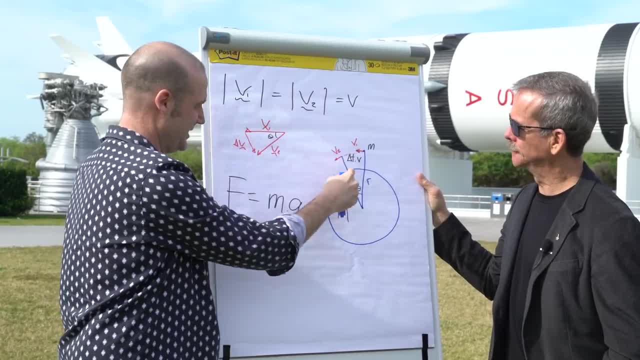 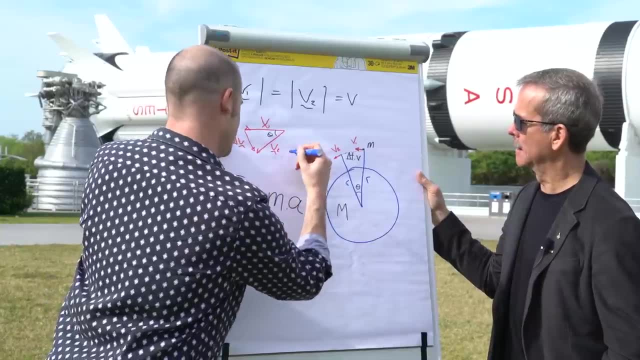 Sure, They're both isosceles, because that length is equal to that length. Yeah, As up here that's equal to that, which means the ratio between any two matching sides should be the same. So the ratio here between change in velocity divided by this side, change in. 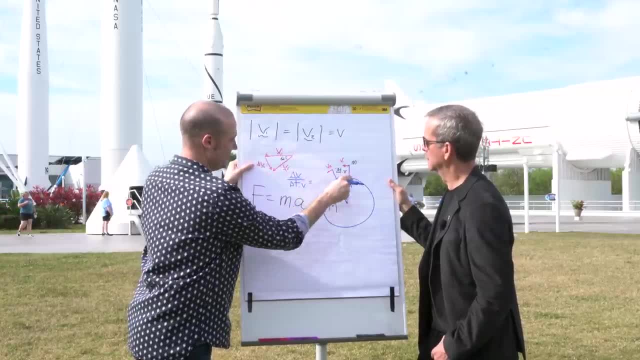 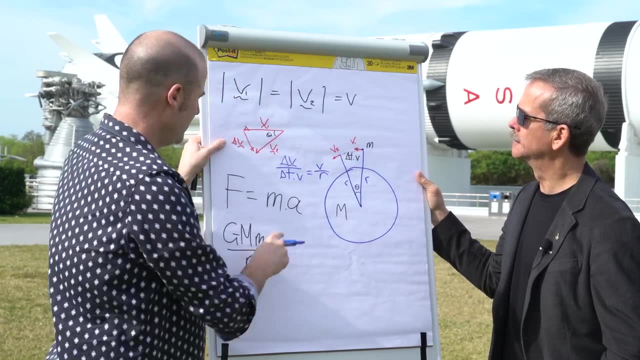 T times velocity equals that divided by that. So that's well, the length of that is just V, divided by the length of that is R. We've got a V down here we don't really need, So we're going to move it over there. So I'm going. 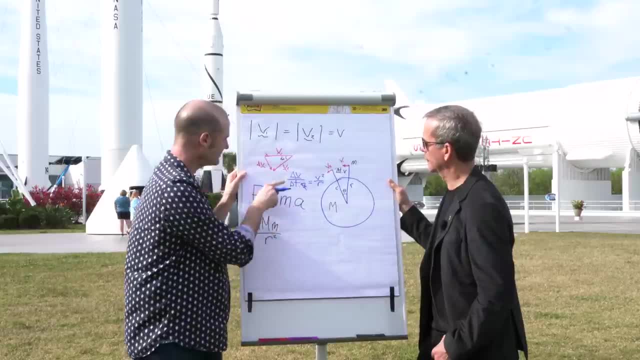 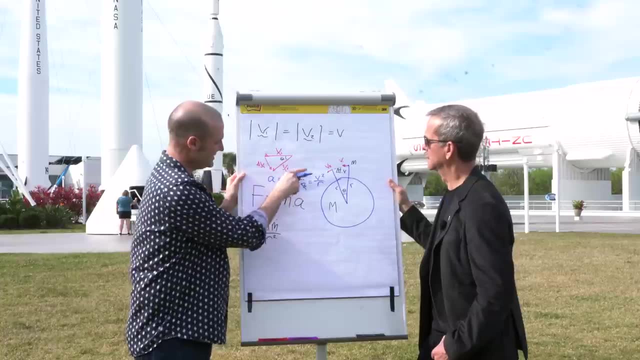 to multiply both sides by V. So that's now over there. Yeah, And dV, dt, rate of change of velocity. that's acceleration. So there we go. So there's. our acceleration is this, which is V squared on R, So I'm going to. 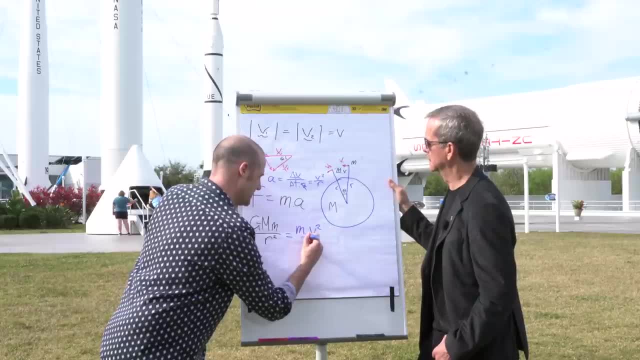 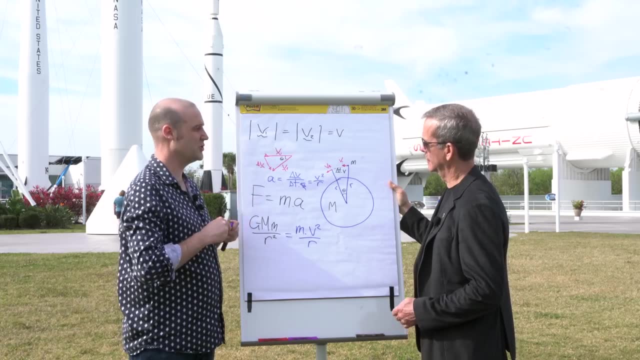 fill that in here. So it's mass times: V squared on R. This is actually just the centripetal force we've worked out. So a lot of times when you see this talk, people just start here. They go, there's your F equals ma, And then you fill this in. That's kind of nice. 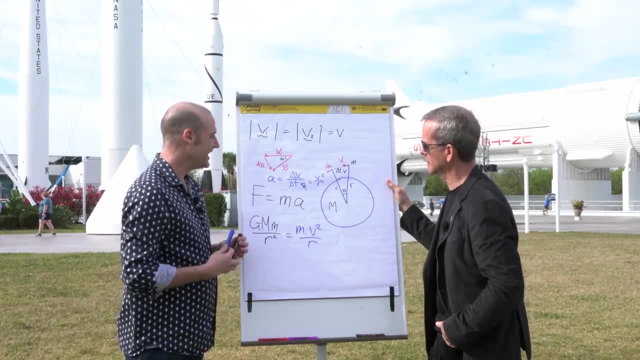 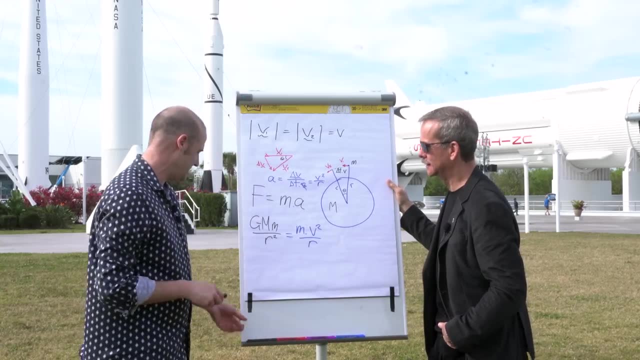 That's beautifully elegant and intuitive. It's so good, So good, And given you were up on this dot, that feels appropriate, Okay. So now let's do the grand finale in Brown, because we can cancel some stuff out. We've got an R down there. 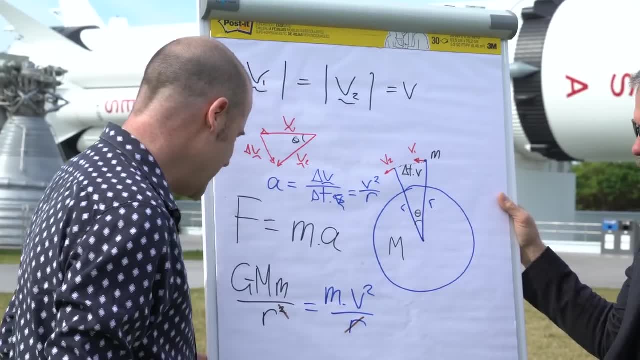 and we've got an R- two R's- over there, So we get rid of one of those. Yeah, Multiply both sides by R. Okay, We can get rid of an M from both sides. So I'm afraid your mass now doesn't matter. 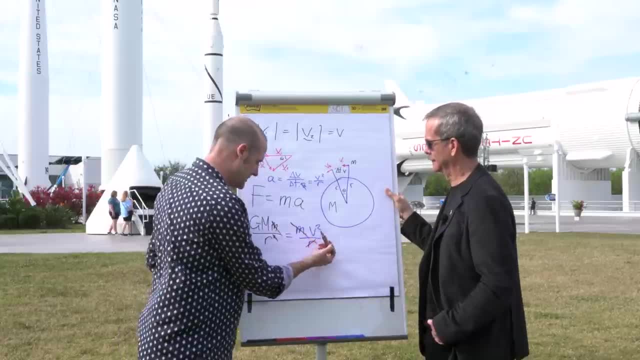 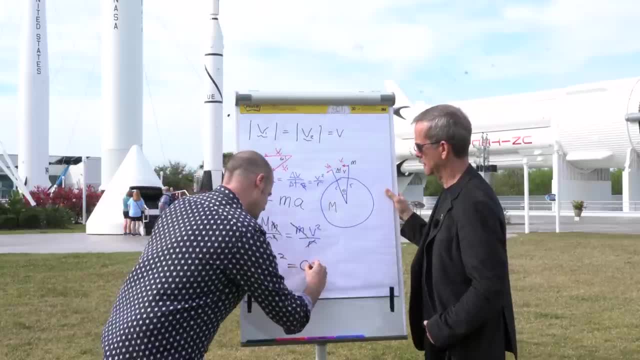 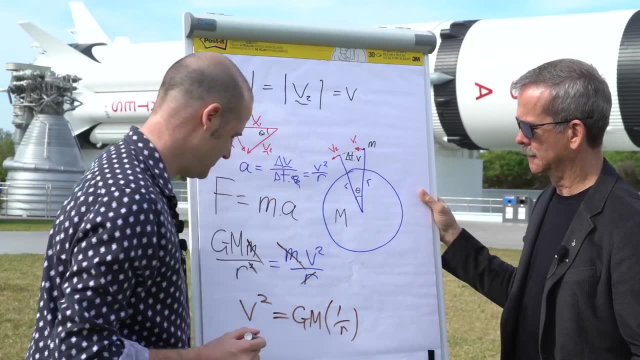 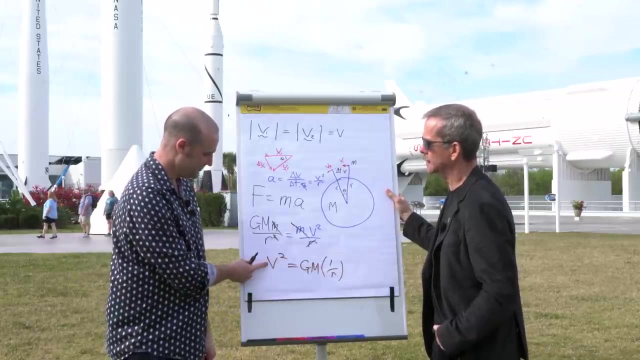 so I've just moved it over here And this is: these are both constants, So I'm going to put G and M over there, And then this is a one over R, Yep, And, and that's it Beautiful. That's our equation. So this basically shows us, if you square the velocity. 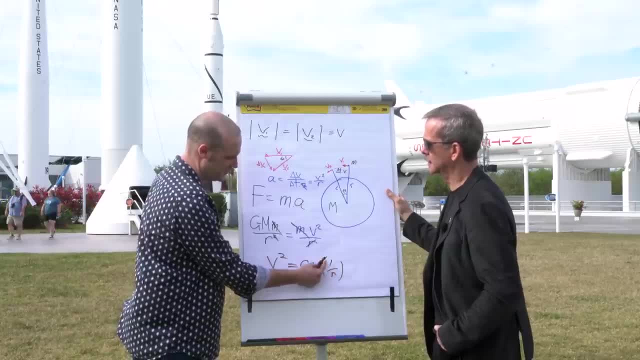 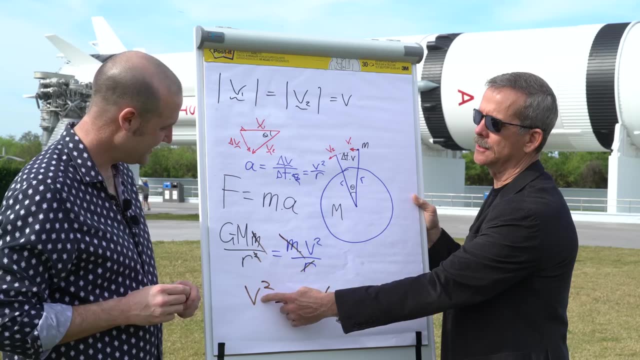 you'll be able to orbit at a height R, And because this is one over R, it's an inverse relationship. You know, what's intriguing to me after this is that the radius you are from the earth determines the velocity you have to go to be. 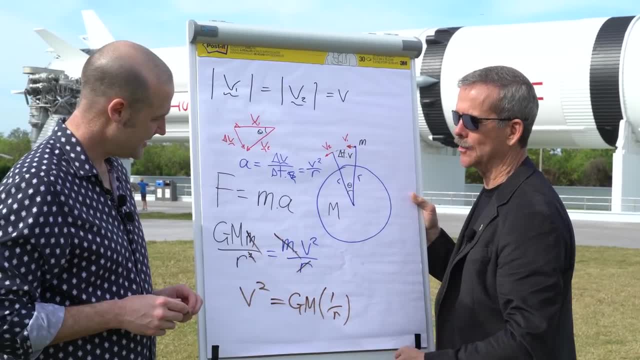 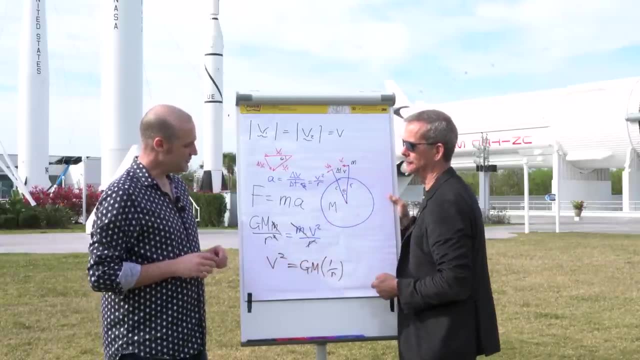 staying in orbit. That's the really key and intriguing thing out of this to me. For every radius from the earth, there is a specific speed that will hold you at that altitude. So if you decide, I want to put either humans in a certain orbit, I want to put a. 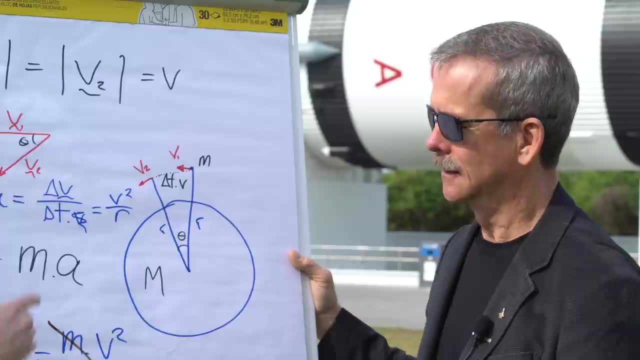 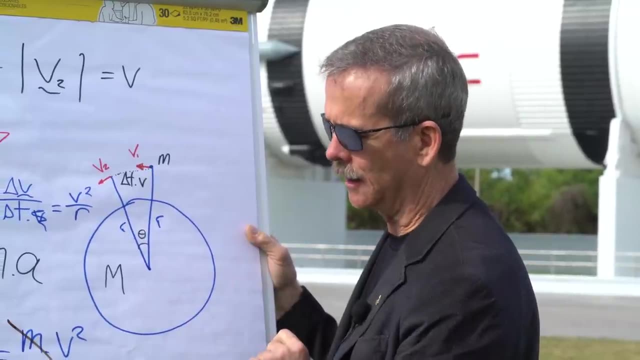 satellite in a certain orbit. you then work out the specific V which equates to that distance, Right, And it doesn't matter what mass that thing is, It's just purely a almost geometric thing: How far away are you? That tells you how fast you have to go. 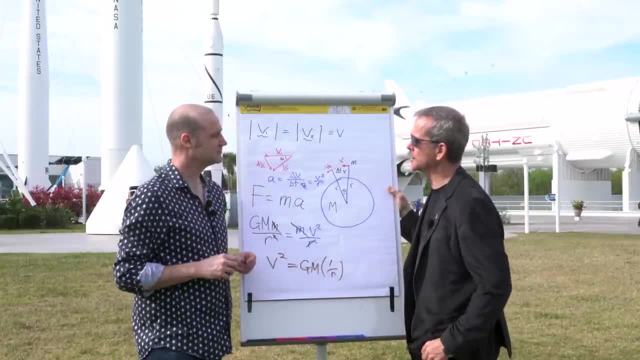 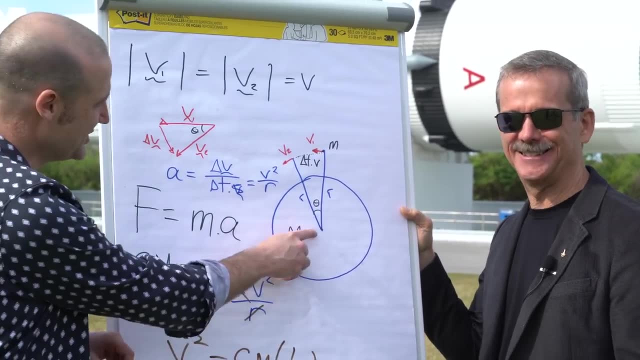 And you were in low earth orbit. Yeah, I didn't get above about 420 kilometers from the surface. So the radius of the earth plus 420.. That's not bad. That's more than most people And the radius is like 6,000 kilometers, right. 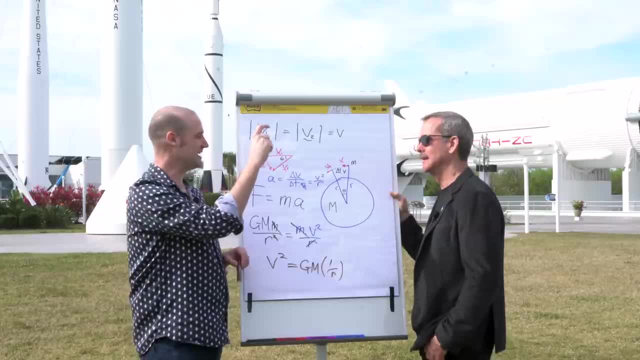 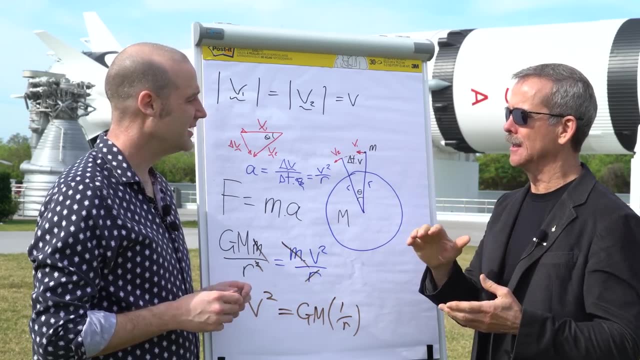 So you're like a tiny like, maybe five, four or 5%. If you were to hold a globe and bring your eyeball down to maybe like a thumb width above, that's how far we were from the surface of the earth. It seems like a long way when you're there. but, but it's actually still quite close. And how fast did you have to go? What was your V for that orbit? Well, depending which units, about 25 times the speed of sound, Mach 25.. If you put it in miles an hour, about 17 and a half thousand miles an hour, about 28,000 kilometers an hour. 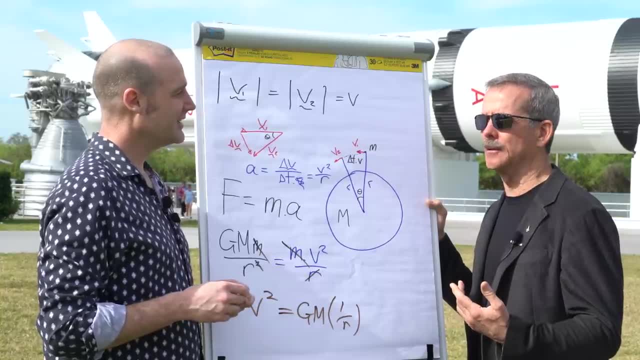 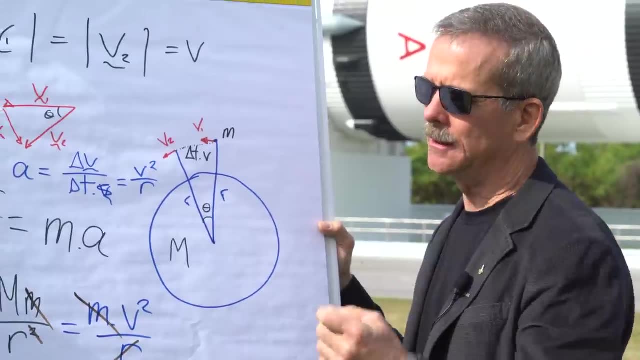 Those numbers are so big. intuitively it's better if you go per second. So about five miles a second or eight kilometers a second In order to stay at that altitude, in that orbit. five miles a second, eight kilometers a second. 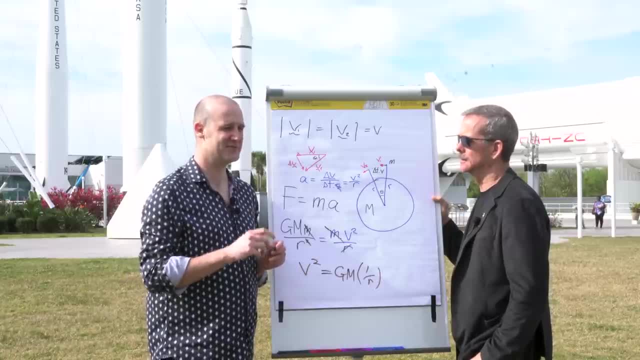 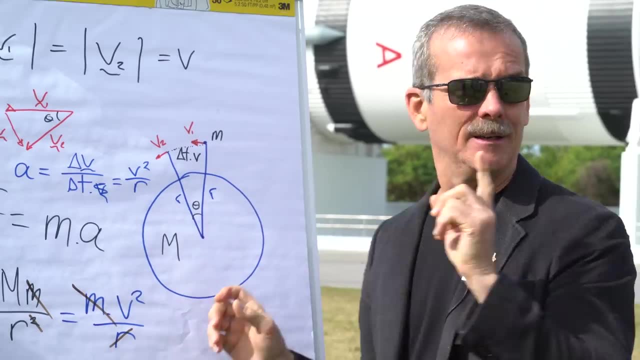 Eight kilometers a second, Yes, That. 8,000 meters every second- Yeah, That's absolutely. Imagine if one of these rockets was right here and one second later it was eight kilometers away. That's how fast we had to be to be that little dot right there. 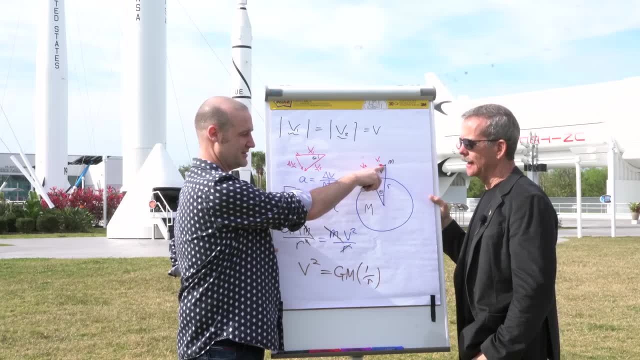 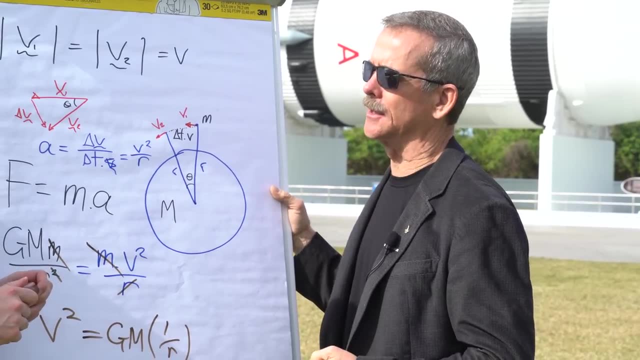 And how long does it take between when you launch and when you get to that orbit? The rockets have to burn and accelerate you up to the right speed and the right angle. It takes somewhere just a little less than nine minutes from sitting here in Florida. 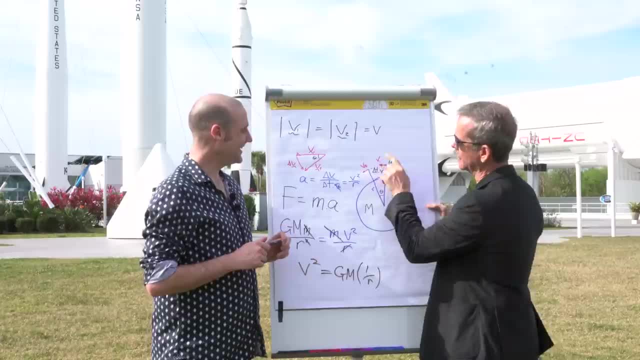 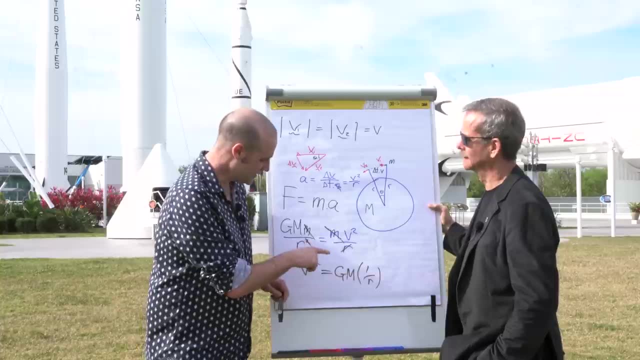 on the pad, laying on your back to the engine, shutting off and being there weightless in orbit A little under the time it takes to drink a cup of coffee. That's absolutely incredible. So, in fact, if people want to give it a go, 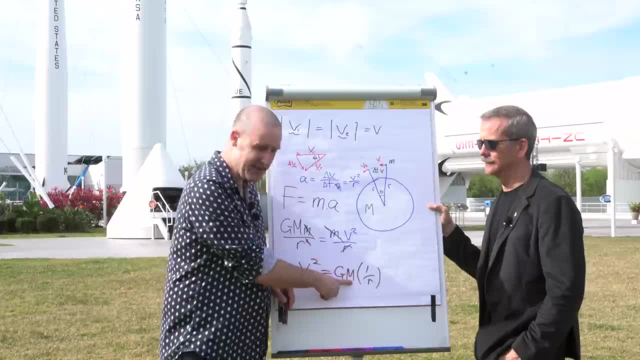 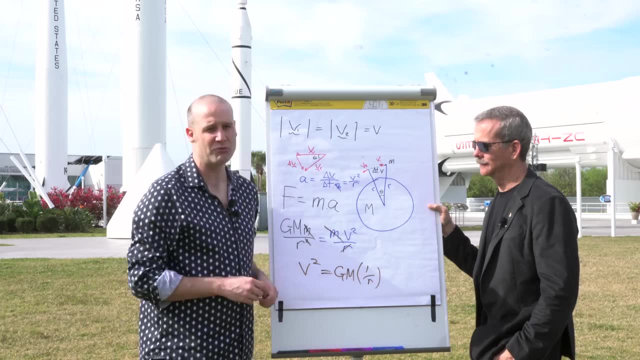 if you get the values for g and m- gravitational constant mass of the Earth- and we've talked through the rough distance up you are- you can put them in and you should get out the other side roughly 8,000, which is 8,000 meters per second. 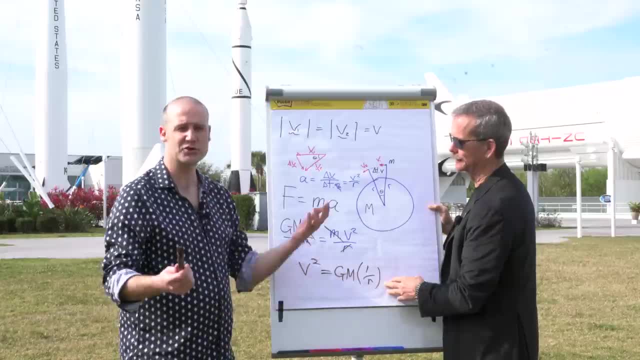 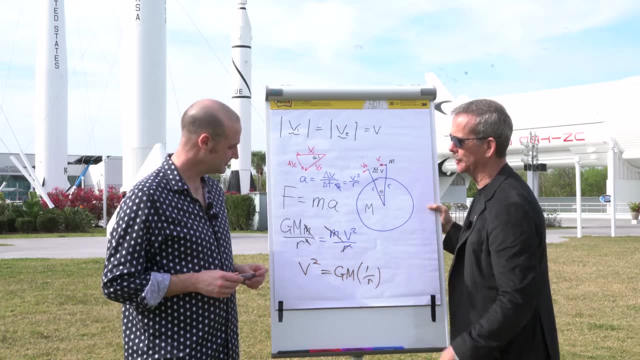 Cool, You could put in the mass for any planet and everything else still works. Oh yeah, That's true. We've not assumed Earth. This could be absolutely anywhere. So you can start to get a bit more out of that. You can start to figure out just how fast you go to go around Jupiter or around the moon or whatever. 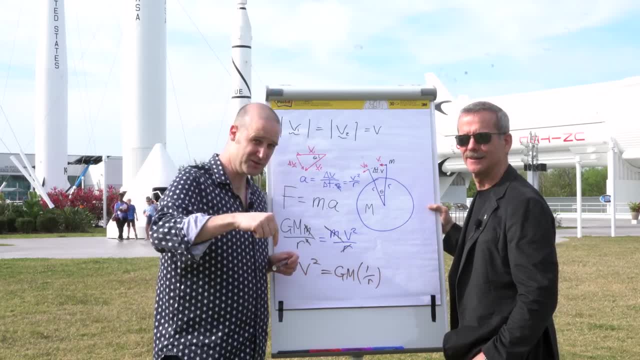 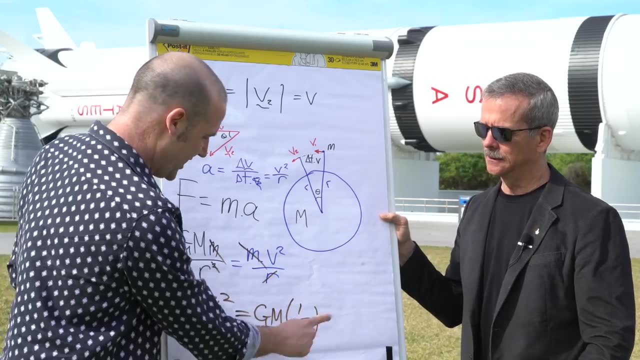 Okay, tell you what. we'll put some free resources in the description below. We'll have a copy of this in case you want to recreate it. But now there's this interesting relationship between how far up you are and its inversely proportion to the speed you're traveling. 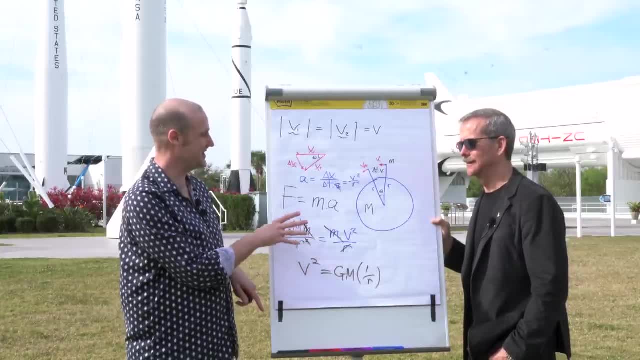 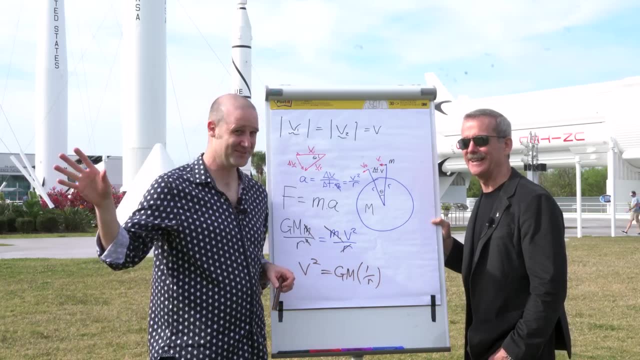 which I suspect has some interesting implications for actually navigating in orbit, And I believe somewhere here is a vehicle that you've flown in orbit. It is indeed. yeah, Atlantis is here. So we're going to go find that and have a chat about the implications of this. 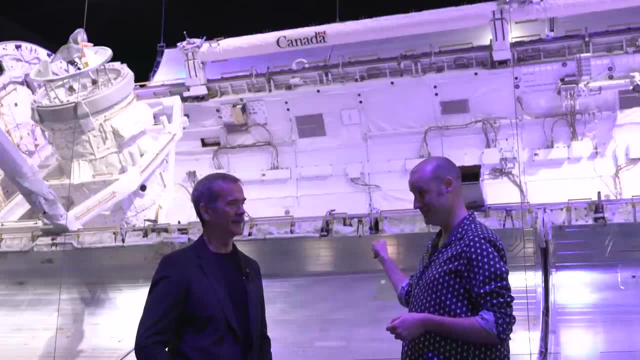 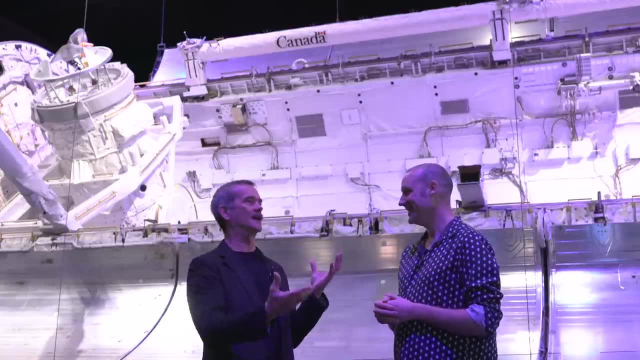 You flew on this space shuttle. I did it my very first time to space. I was part of a crew of five people and we took this vehicle, flew it up and docked with the Russian space station Mir, And that's not like an automated process. 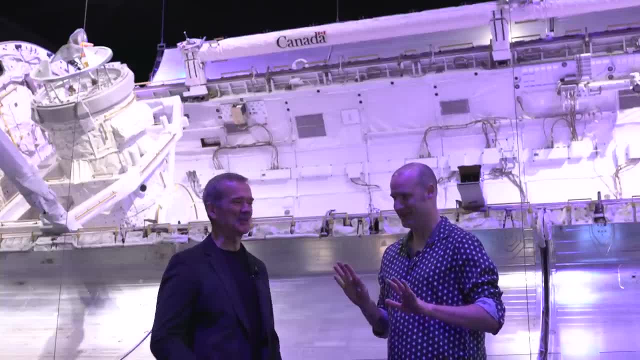 You don't just hit the dock button And it all happens. No, there's no standard orbit, Mr Sulu. It's all sort of manual. I mean, you have primitive computers on board. a huge amount of help from Earth. 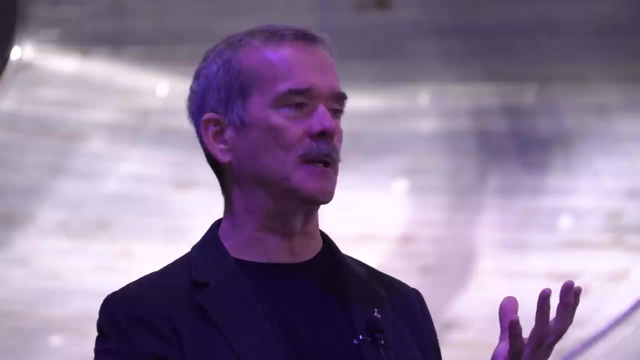 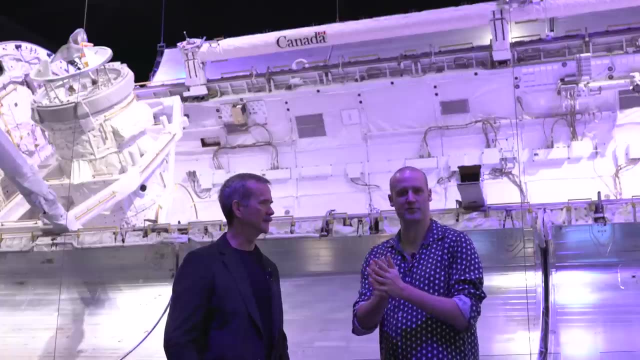 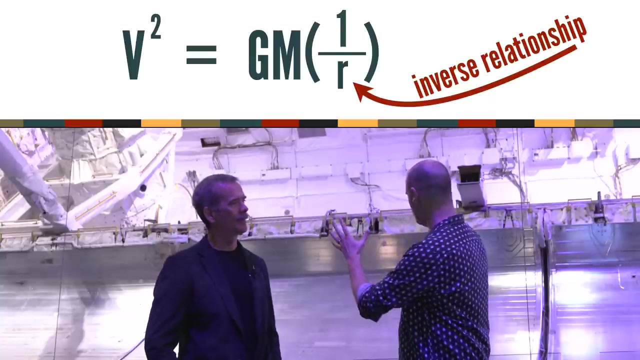 but primarily flying a spaceship to dock with a space station is a manual operation, especially with something as big and ponderous as a spaceship. So I've always known on paper: a lower orbit, higher velocity. higher orbit, less velocity. What does it actually mean if you're trying to maneuver this? 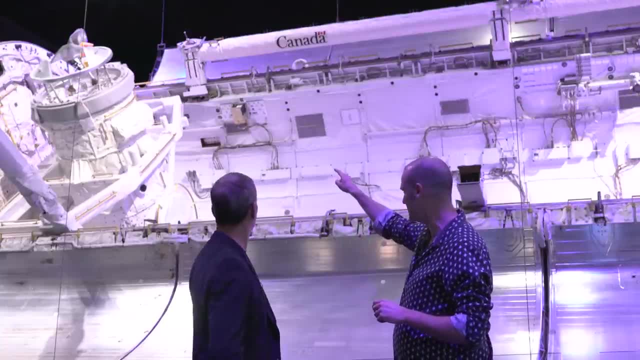 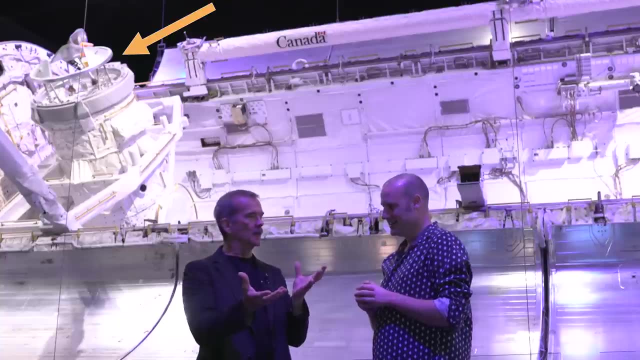 and you're going to connect that bit. It's a very specific bit on another space station. So picture this: Matt, You have to dock that docking system to Mir. You have to do it inside a two-minute window because you have to be over the right part. 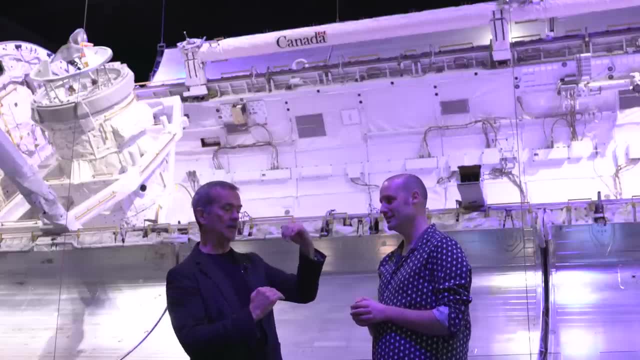 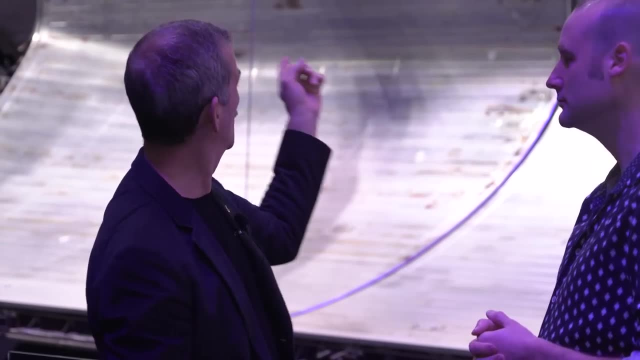 of the Earth for communications, You have to do it at exactly the right speed. If you come in too fast then you'll break Mir and kill the three people on board. If you come in too slow, then the springs in there will bounce you off. 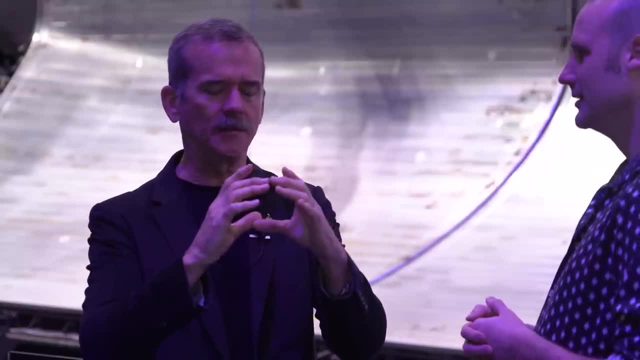 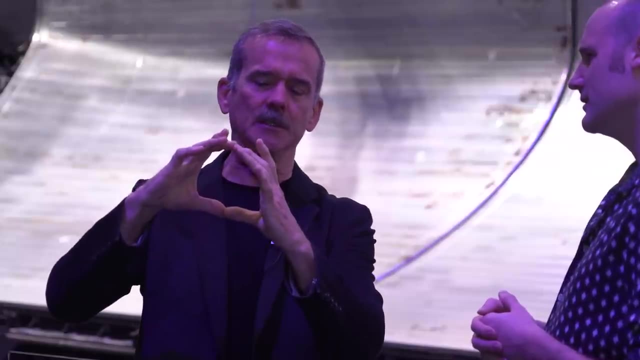 And plus you've got to hit it exactly in the center, because if you hit a little bit off center the mechanism will bottom out and break. So our target was about as big as maybe, a coffee saucer. So all those constraints and you're flying it manually. 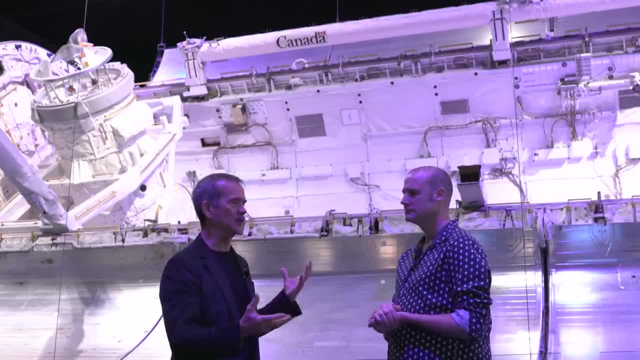 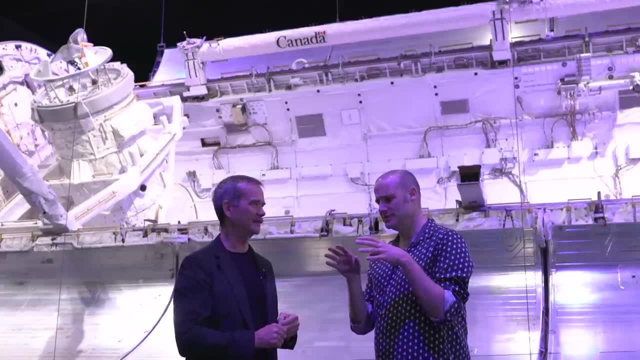 And so an extremely difficult ballet to make all those things happen at once. And, as you say, you're trying to negotiate orbital mechanics while it's happening. So what are you doing? Are you just using the thrusters, or do you have to take into account if you go up, or 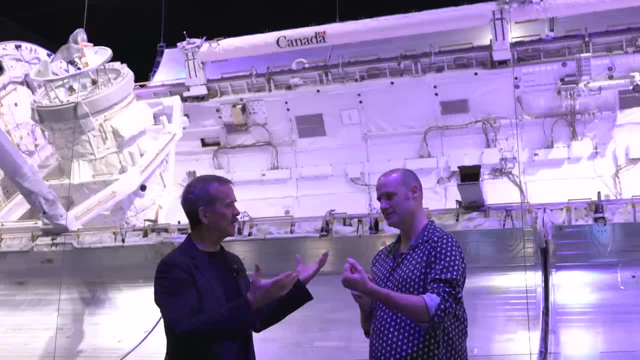 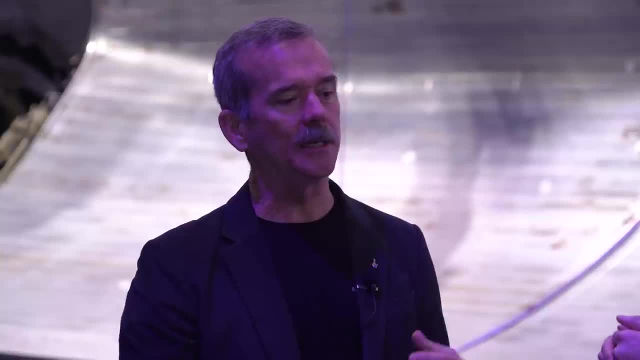 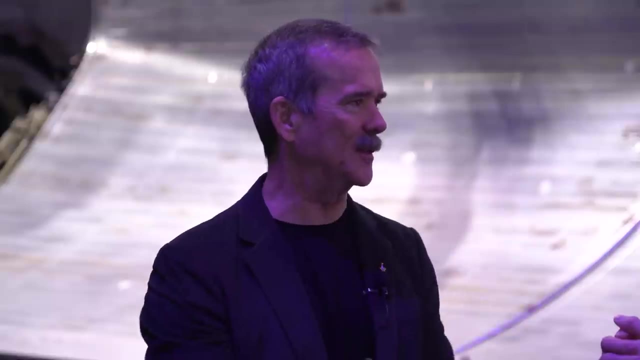 down, your speed's going to alter. We try and solve that mental problem of the difference of speeds with different orbit heights by breaking your docking into phases. When you're far away you hardly even acknowledge that the Mir is there. You're just a vehicle going around the world and you're going to change your orbit. 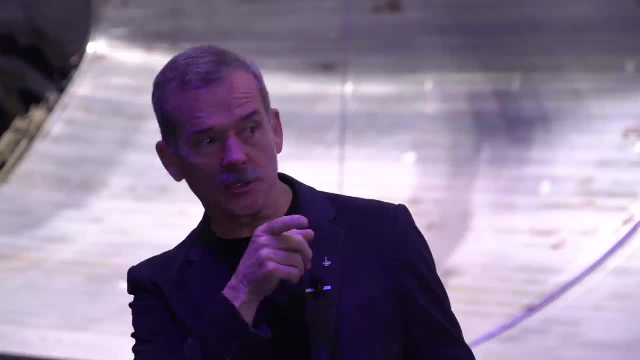 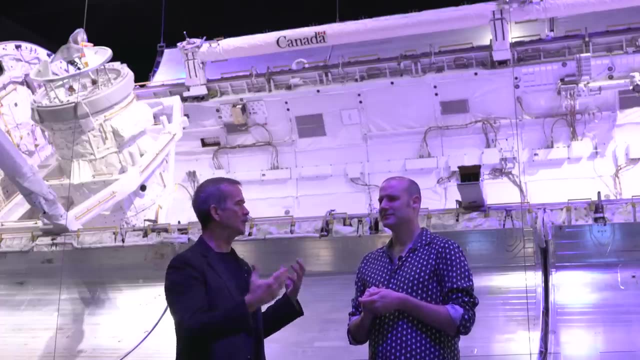 And so if you're going this way and you fire the big engines to accelerate that way, then the energy is going to raise your orbit. You're going to end up in an orbit that is further from Earth, and once you get up there, 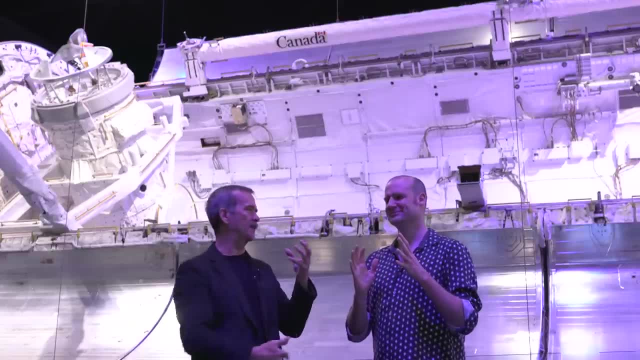 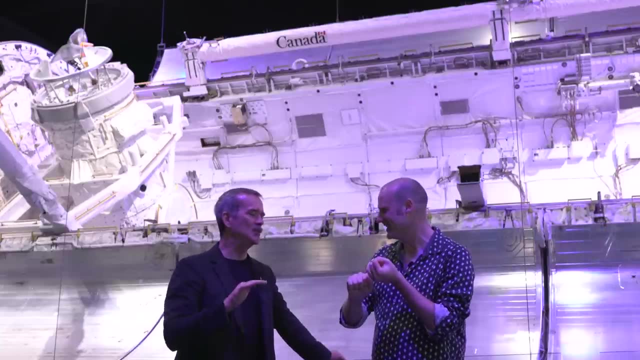 you'll be sort of going at a slower speed, Like the moon takes a month to go around. So you fire the rockets, You don't speed up. Well, you do sort of accelerate forwards, but that energy ends up because you're going. 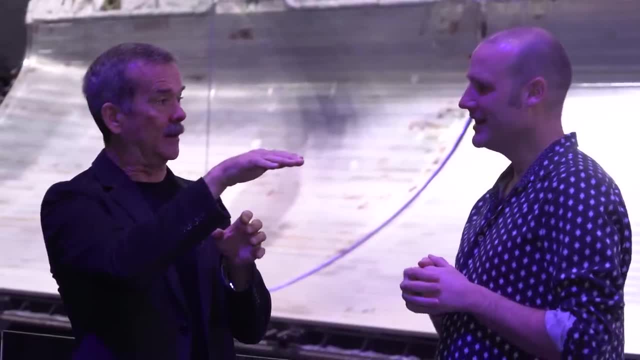 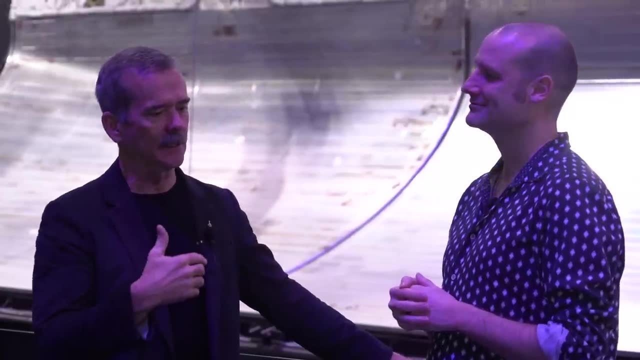 around the world. that energy sort of takes you away from the world a little higher, right, Until everything balances back out. And once you're higher and balance out- now in fact your speed is lower- It turned sort of that kinetic energy into potential energy, so now you're further away. 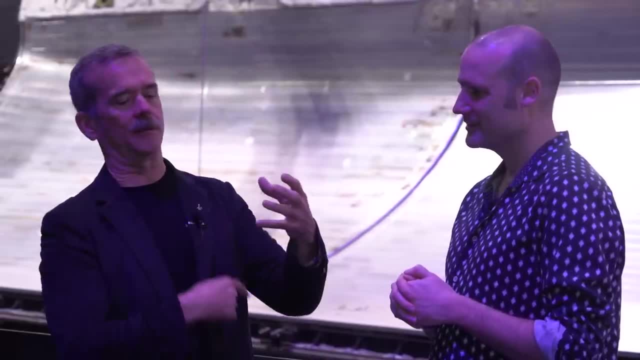 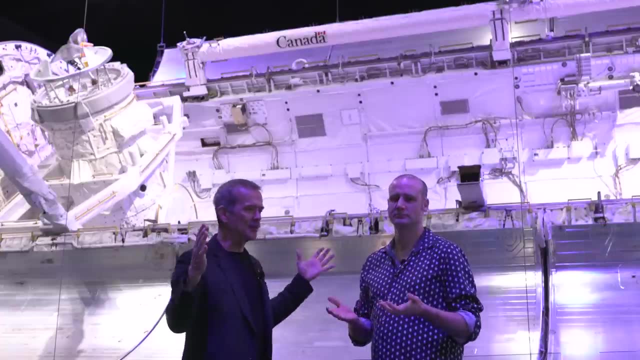 Yeah, So the moon is way out there. It takes a month to go around the world, And like a ball and a string, the shorter the string, the faster you have to spin it to keep the ball going, And so your string's just getting shorter and shorter. 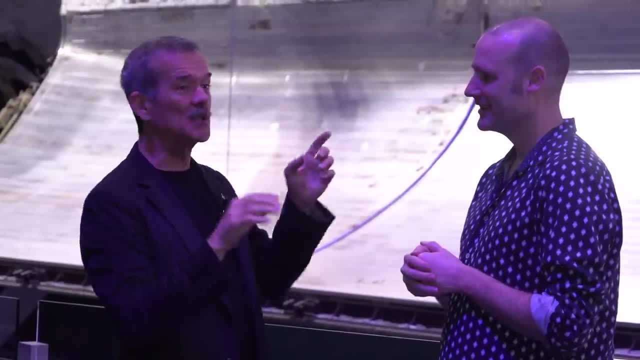 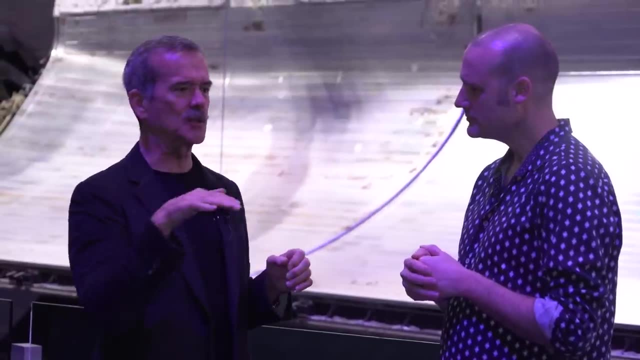 So you fire your engines and you coast to where you are. But once you see Mir- and now you fire your engines to get higher- suddenly it becomes non-intuitive, because we fire our thrusters to go this way and we're watching intently. 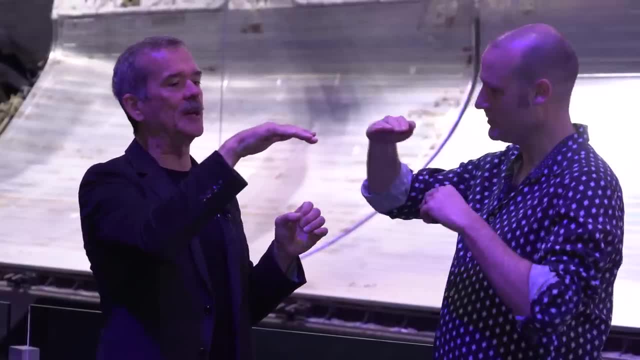 at Mir and we get a little closer to Mir, because we move up from underneath it and then we start drifting back Because you're higher than it, Because we're higher, and now we're slower and we're drifting back. 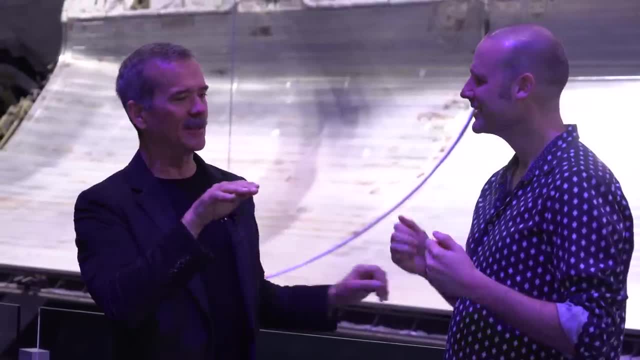 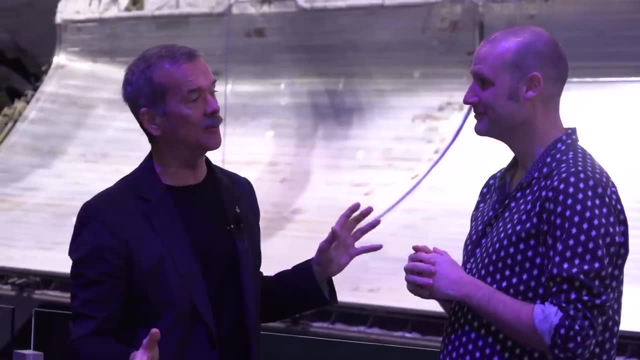 So we're still playing with our speeds as we go until we finally get close enough that we say, OK, we can no longer pay attention to orbital mechanics. Now we're just going to brute force it. We call it proximity operations or prox ops. 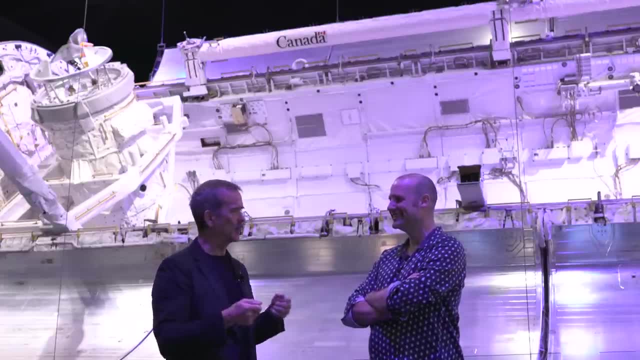 Proximity operations And once you're in prox ops, all you do is say we're a little forward, we're a little aft, and just keep firing the thrusters to hone it in so that you can dock under exactly the right conditions. 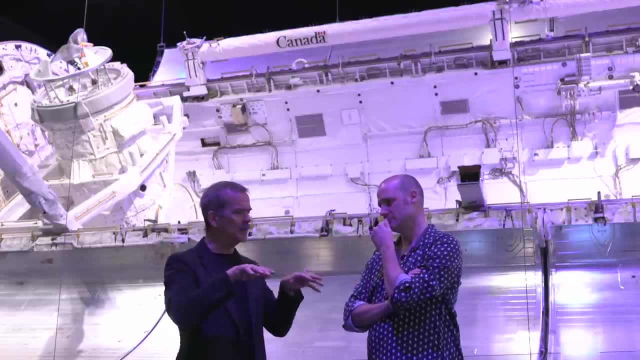 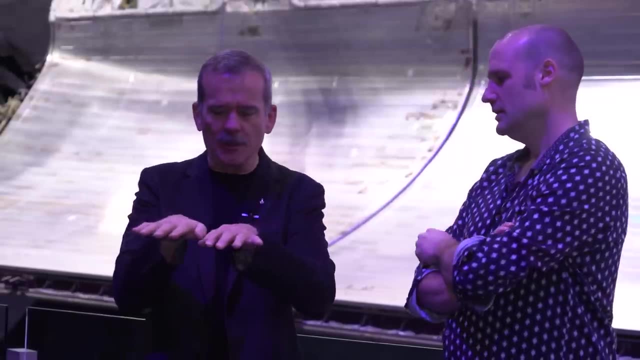 So you're just compensating on the fly. It's sort of like if you were driving two boats across a lake and you're trying to touch maybe two parts of the boats to each other very carefully. From a distance you'll just sort of make a rough guess on where to set your throttle. 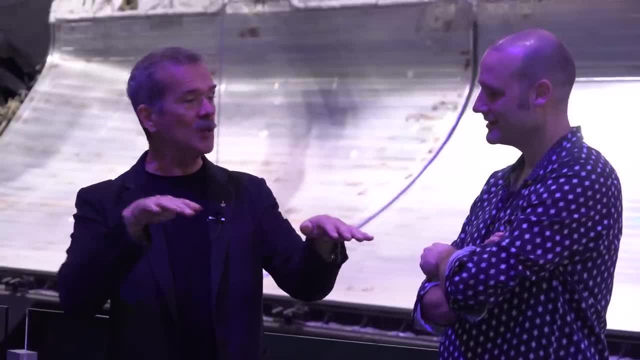 And you might even just set the throttle and not even move it for a while. just catch up. Then, as you get close, you're going to fine-tune your throttle a little, but once you're nudging up against that other one, you're going to be all over the throttle and the steering. 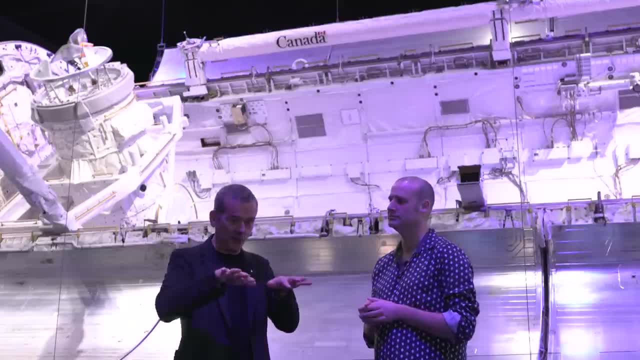 wheel and you won't care about the current or the wind or the surf, you're just trying to get docked, Sort of like that. One of the things I'm doing working out- and I know I'm near the answer is just that that's. 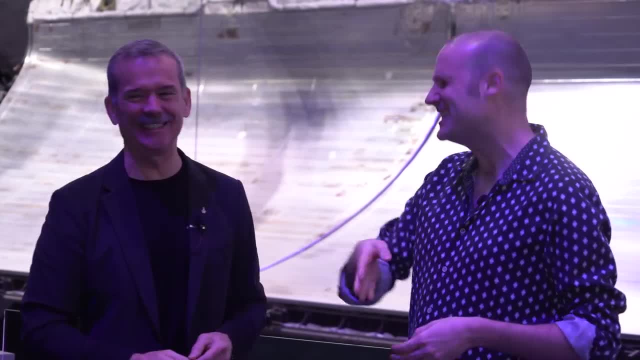 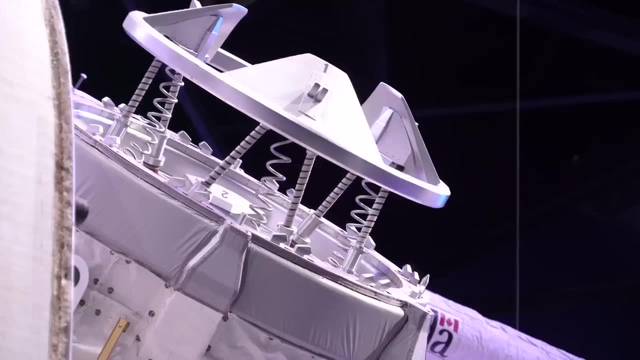 my proximity operation zone where I'm just kind of: yeah exactly, you run a simulation, you end up where you're meant to go, So excellent. thank you so much for joining us and having a chat. Well, that's a lot of space maths. thanks for watching the video. 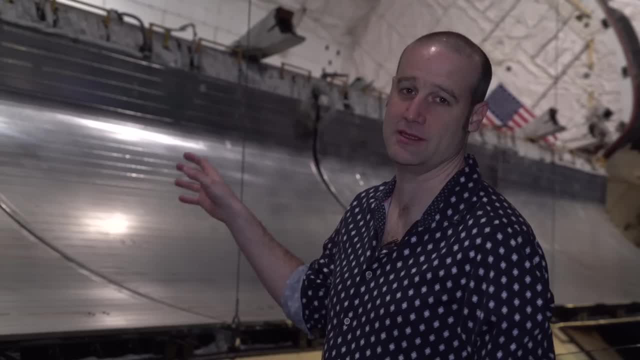 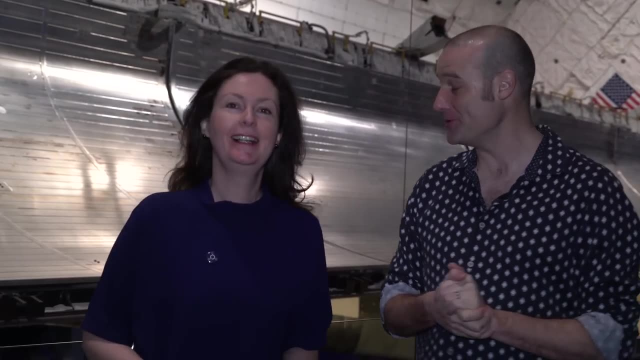 There is also some engineering and some science which goes into something like this. So, as well as my videos, you want to check out the videos by Professor Lucy Green over on the Cosmic Shambles Network. Yes, We've made some fantastic videos looking at what goes into making the Space Shuttle fly. 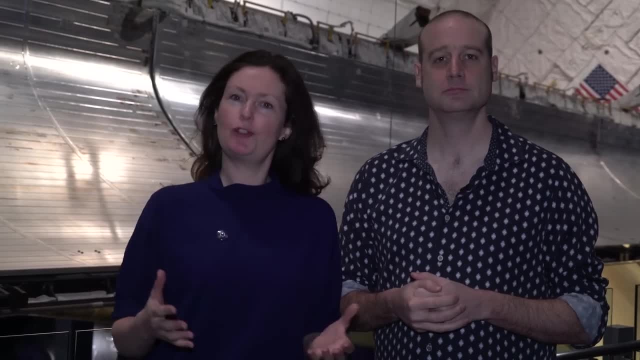 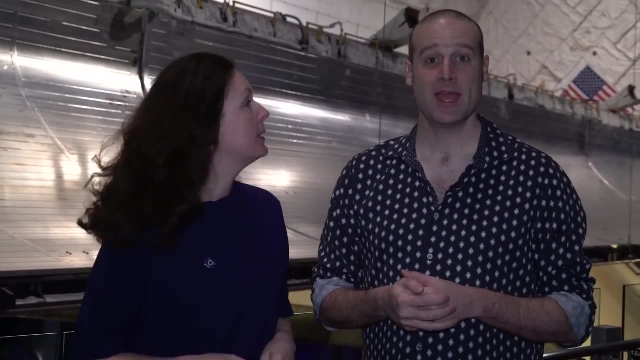 the work that's done on it. a bit of space weather from an astronaut's perspective as well. so huge thanks to Chris Hadfield for giving up his time to tell us about this amazing technology, And we'll have links to those below. it was actually the Cosmic Shambles Network who put 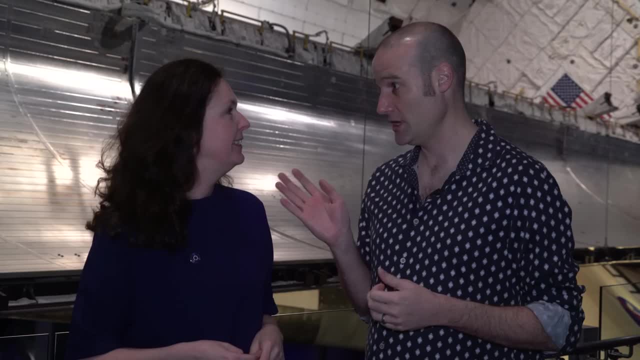 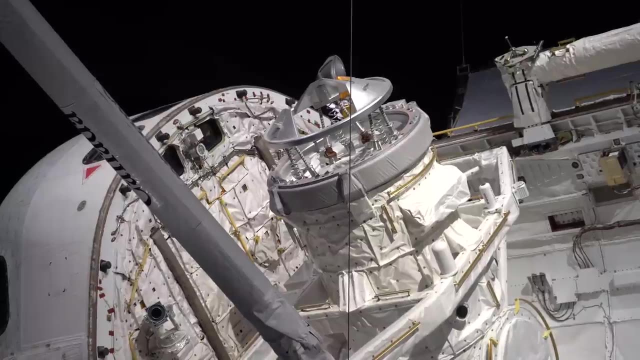 this whole trip together. so huge thanks to them, Chris, of course, and let's not forget that the Kennedy Space Centre and NASA were also slightly involved. Thank you so much for watching and I'll see you in the next video. Bye. Bye, Bye, Bye.